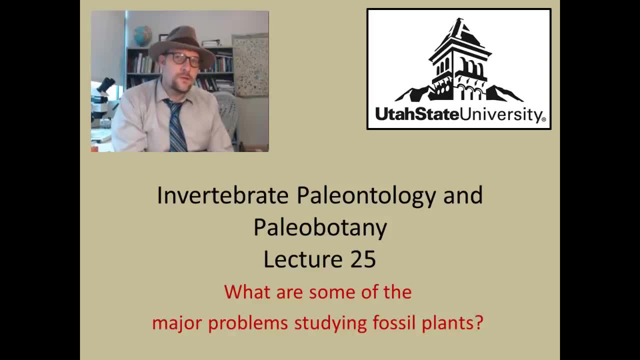 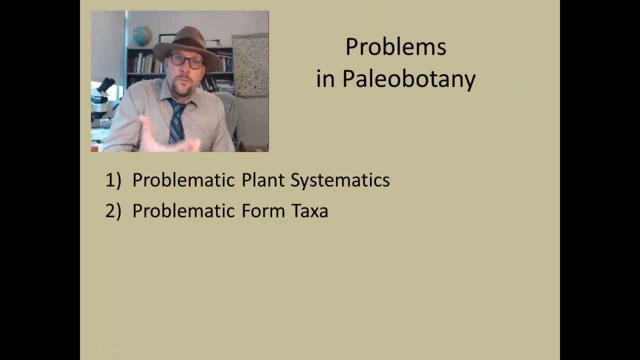 Welcome to Invertebrate Paleontology and Paleobotany at Utah State University. This is lecture 25, where we will talk about some of the problems in studying fossil plants. And oh boy, we have some challenges ahead of us. There are two major difficulties in studying fossil plants. 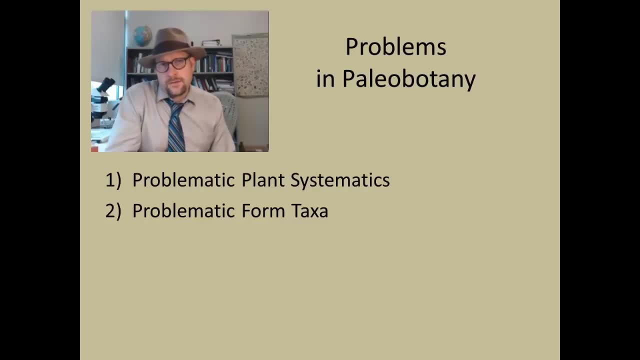 First, the systematic relationships of plants and very primitive protists, photosynthesizing single celled eukaryotes. It is a bit of a mess. It used to be that all of these single celled organisms were all stuffed into a single kingdom. But clues from molecular phylogenies. 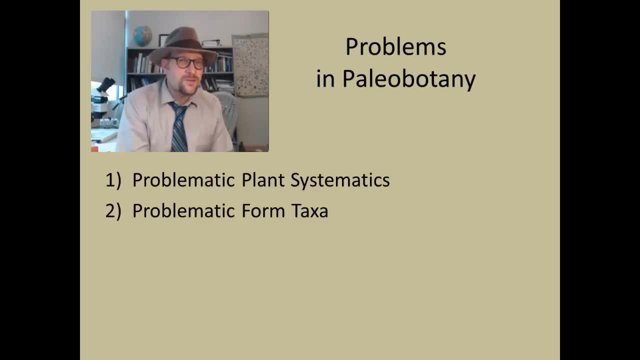 have caused us to realize that many of these groups probably deserve their own kingdoms. The other problem with studying fossil plants is that they are not just a single body. Plants have leaves and roots and trunks, They have pollen, seeds, even different sexes, and some even have complicated life cycles. 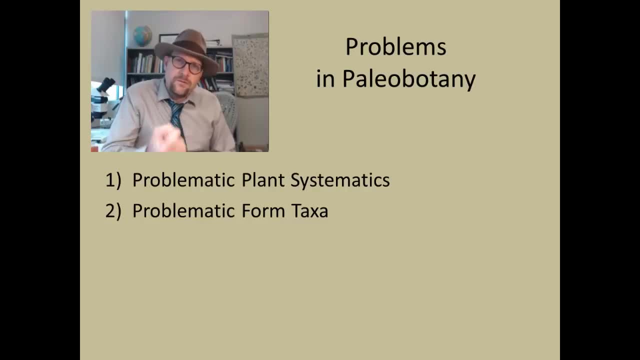 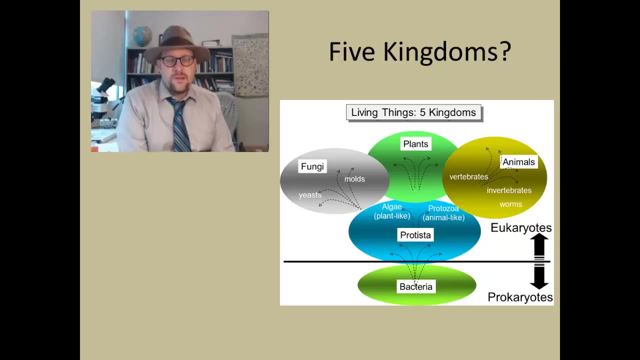 It is difficult to pick up a single fossil and have a good idea of what the entire plant actually looks like, So paleobotanists have to use form taxa. The old system of five kingdoms of life might have been something that you were introduced to. 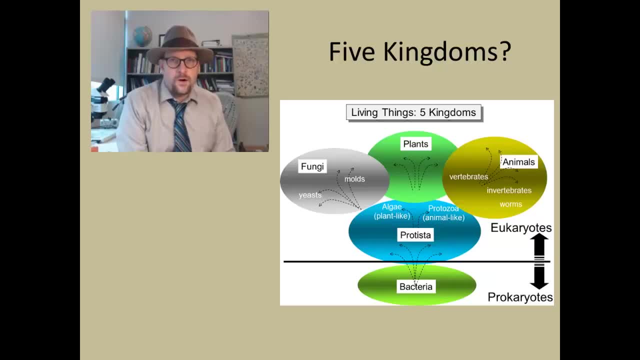 When you were taking high school. Alright, let's get into it. high school biology: There are the animals, the plants, the fungi and the protists, the single celled eukaryotic organisms and the bacteria, so five kingdoms. 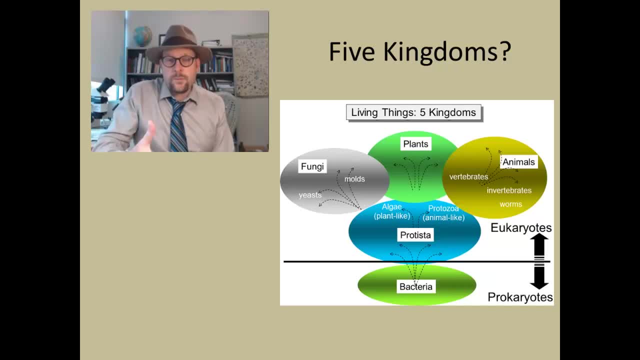 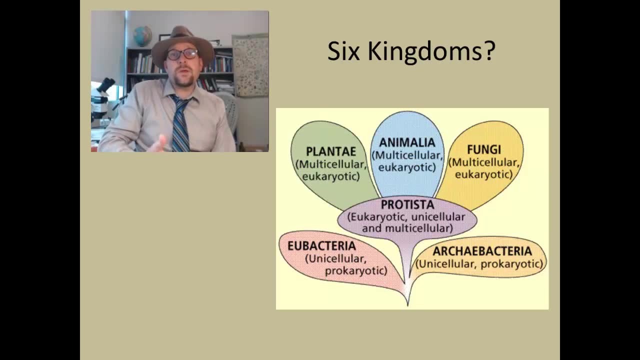 Hence all eukaryotic single celled organisms are placed within a single kingdom. More recently, folks studying bacteria decided to split bacteria into two kingdoms. The Eubacteria and Archaobacteria are Archaea with six kingdoms, But today things are getting a little freaky. 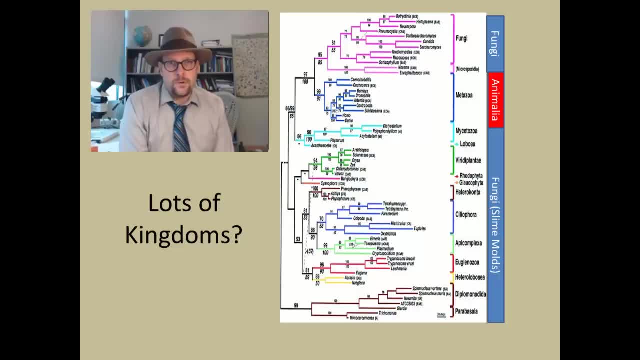 For example, if we look at a cladogram of fungi and animals, we note that fungi represent two groups, one more closely related to animals and the slime molds being more distantly related. So one could argue that fungi should be more closely related to animals. 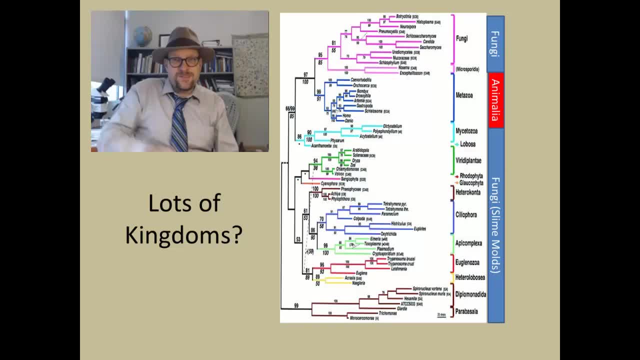 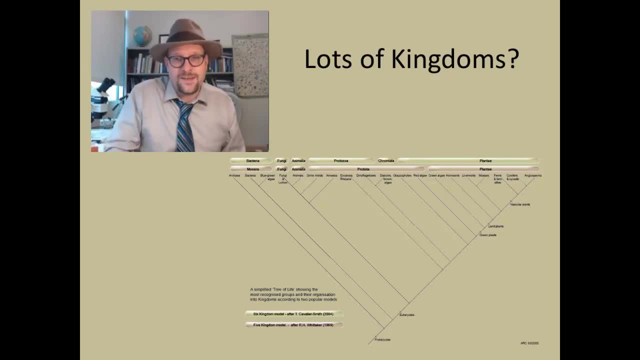 The real big kicker is, if we start looking at single celled eukaryotes and their phylogeny, Some of these groups are going to be more closely related to animals and fungi, while others are going to be more closely related to plants. 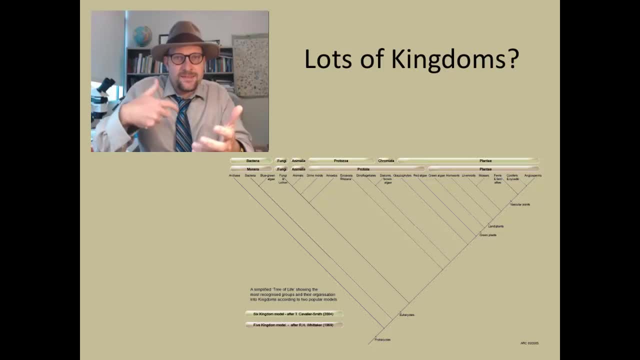 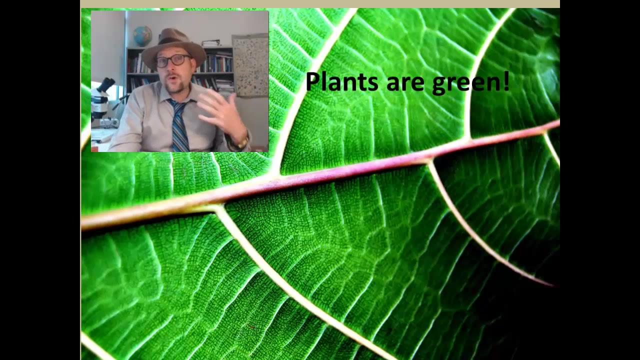 Hence the protista doesn't seem to be representing a single monophyletic group, but a polyphyletic group. Eek Oh man. If there is one thing we can all agree on, it is that plants are green, And they are green because they contain chloroplasts. 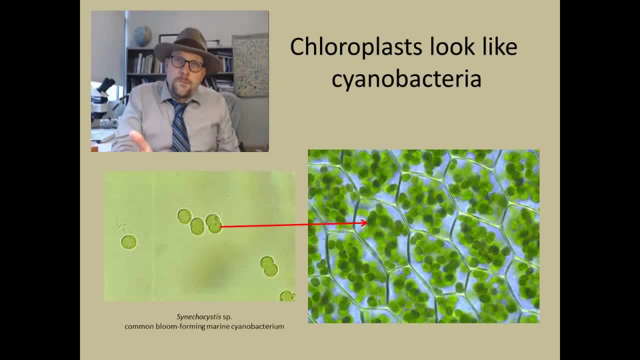 These organelles allow for photosynthesis. Some prokaryotic bacteria also have chloroplasts- the blue-green algae, the cyanobacteria- And it is thought that the chloroplasts that are found in plant cells are basically the cyanobacteria that have been incorporated into the eukaryotic cells of plants. 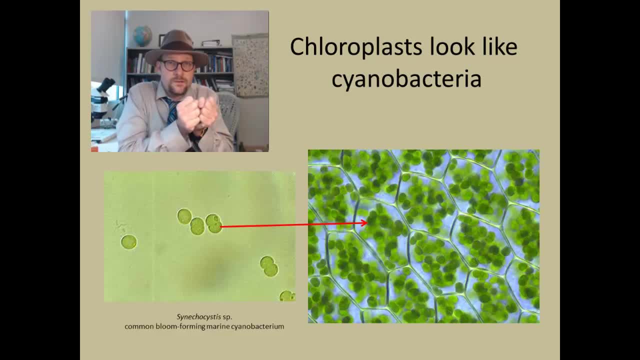 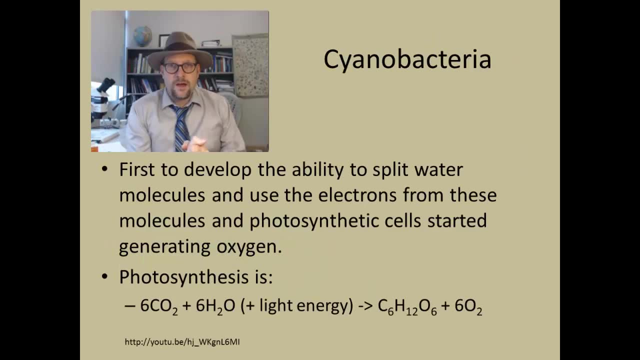 This allows both the cyanobacteria and eukaryotic organisms to have chloroplasts and to do photosynthesis. Photosynthesis is a pretty complex chain of chemical reactions that basically take carbon dioxide from the atmosphere, combined with water and photons- light waves- to create. 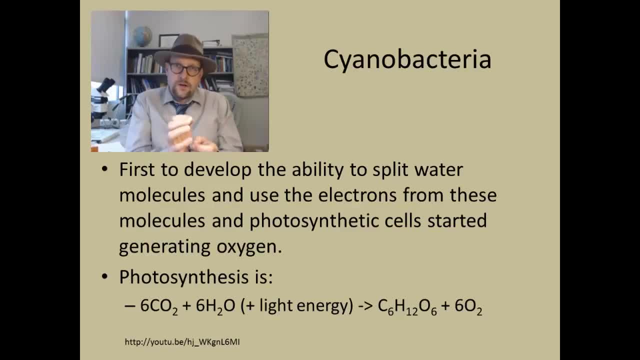 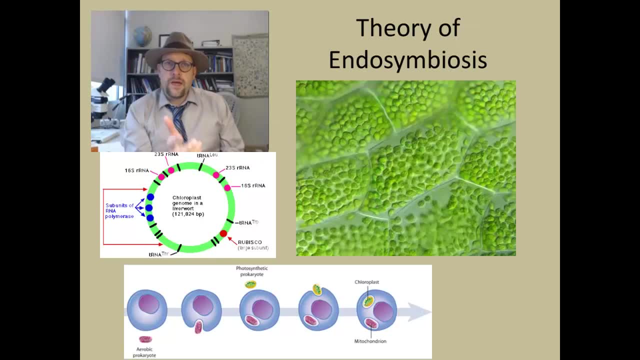 sugars and oxygen. The oxygen is a waste product, while the sugars are used as a source of energy. The strongest evidence that chloroplasts are actually invaginated cyanobacterial cells is the fact that chloroplasts have their own DNA, which is arranged in a circle similar. 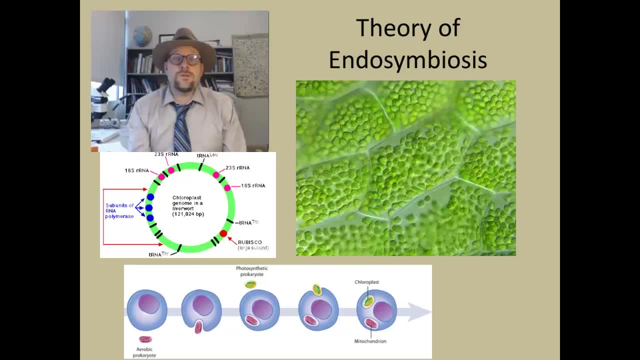 to what you find in prokaryotic cells. The endosymbiosis hypothesis is that early eukaryotic cells are formed by the use of chloroplasts. The eukaryotes incorporated protokaryotic organisms within the cell, giving them a 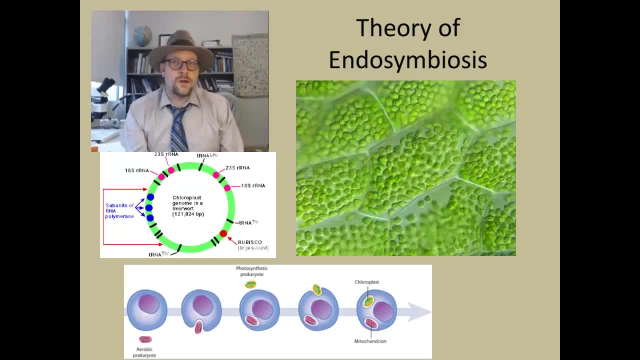 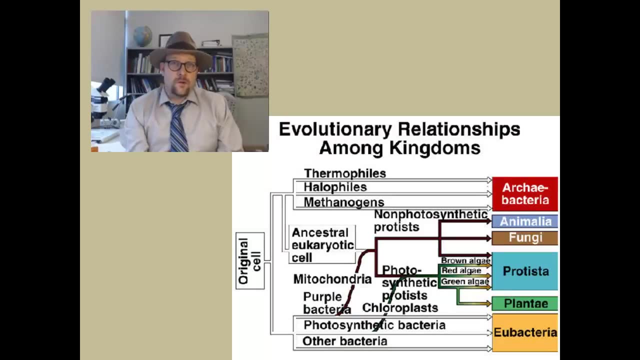 superpower of photosynthesis, They also incorporated mitochondria allowing for cellular metabolism. Now, what is peculiar is that the groups that gain the chloroplasts go on to form- the groups that include plants- while the eukaryotes that just have the mitochondria go on to form. 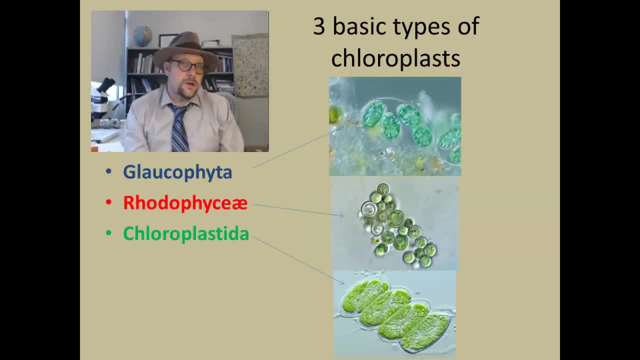 the fungi in animals. Botanists have been looking at chloroplasts in plant cells, as well as various single celled photosynthesizing groups, and they are realizing that there are many different types of chloroplast organelles and that many of these different organisms came by. 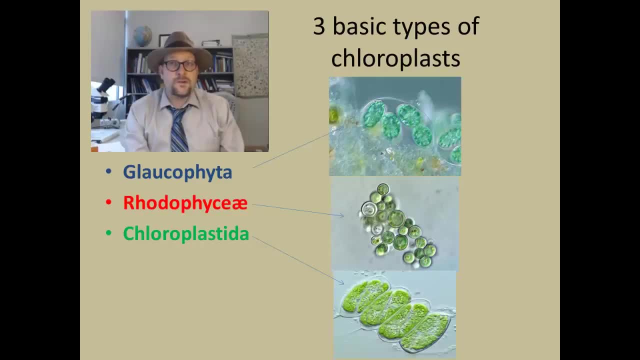 these separately, with separate events. So, for example, there is a blue glaucophyllate found in some primitive algaes, The red rhodophyllate found in red algaes And the chloroplastate, which is a group of chloroplast cells that are found in green. 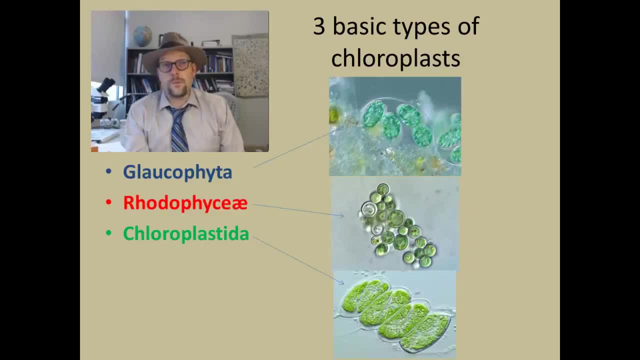 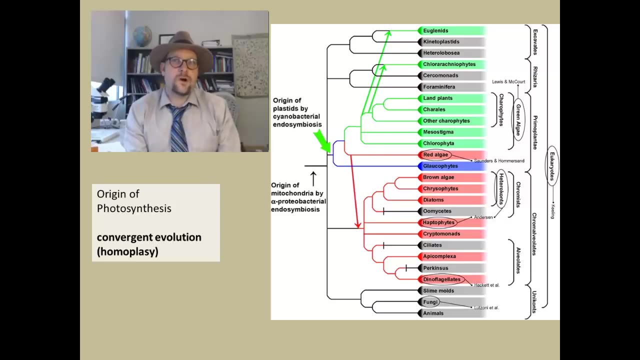 algae and plants, So many of these might have different types of chloroplast organelles. Now, to make things a little more complicated, these different types of chloroplasts were acquired in different amounts and quantities. It's like these cells were filling their pockets with different types of chloroplasts and using 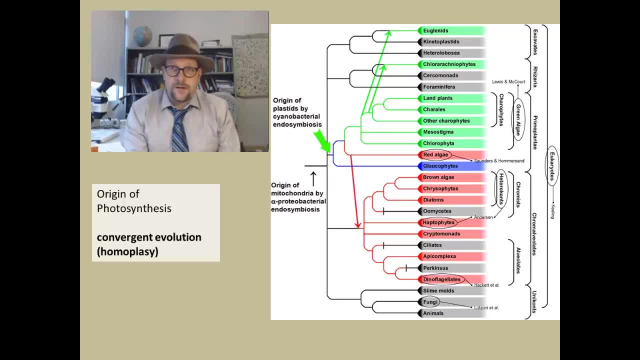 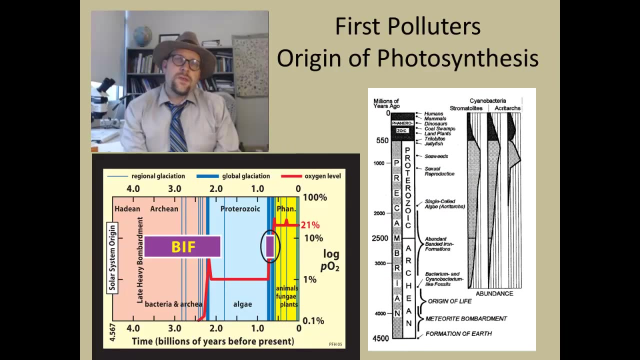 them when needed. Sometimes chloroplasts were stuffed together in such that you get these double or triple cellular walls forming. So this character is likely a really complicated character that probably evolved many times across numerous different lineages. Now the one thing that everyone seems to agree on is when the origin of photosynthesis occurred. 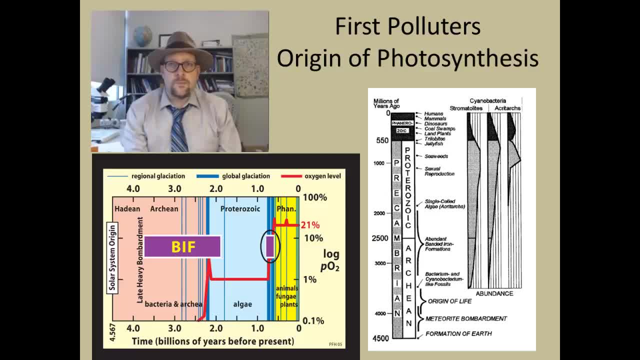 And it really took off. and this is during the period of time between the boundary between the Archean and the Protozoic, when the atmosphere began to be filled with oxygen. Hence, these early single celled photosynthesizing life forms were the first polluters of the 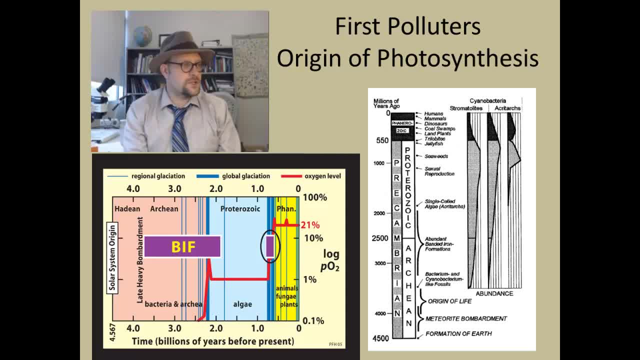 planet and we've been breathing in their pollution oxygen ever since. The evidence for this change is in the fact that banded iron formations, BIFs, are not found during the Protozoic, Except for some brief intervals. So what is the difference? 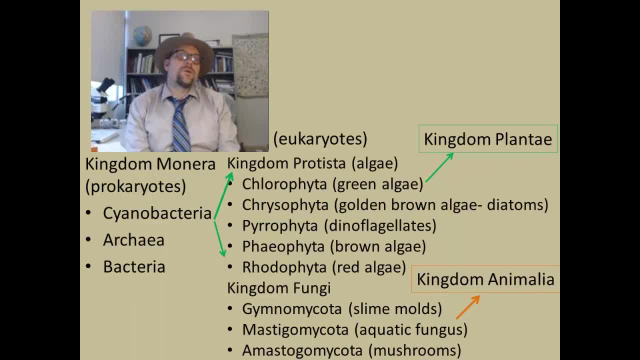 Well, in this class we will try to keep all of this simple, as simple as we can. So here is the classification of the various groups of life. We have the Prokaryotes, the Monotra kingdom, which includes Cyanobacteria Archaea and 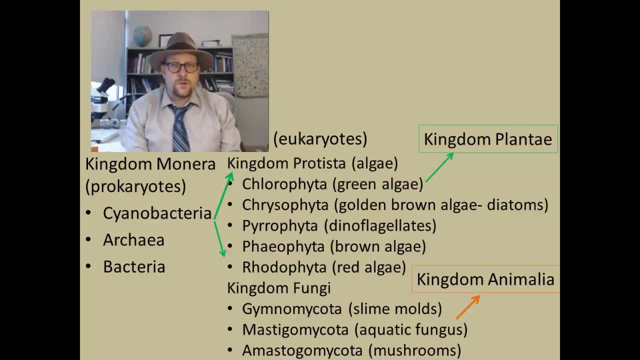 Eubacteria. Then we have the Eukaryotes, which include the Protista, the chlorophyte green algae, which includes the Diatoms, the Pyrophyllite, the Ditaflagylates and the Charophyllite. 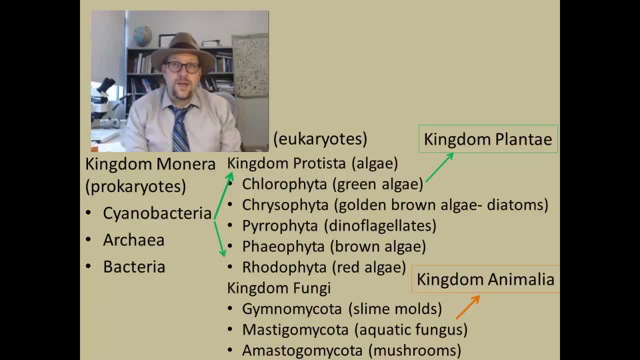 the brown algae and the Rhodophyllite. the red algae Plants are most closely related to the green algae. On the other side, we have the Eukaryotes that lack chloroplasts. these include the Jimyamakato. 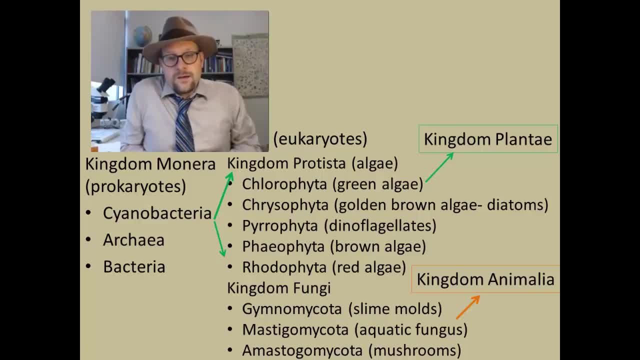 the Slymold's, the Masiomakato, The aquatic fungus, and the Amastogomakata, the mushrooms. Of these, the Amastogomakata, the aquatic fungus is the one that appears to be the. 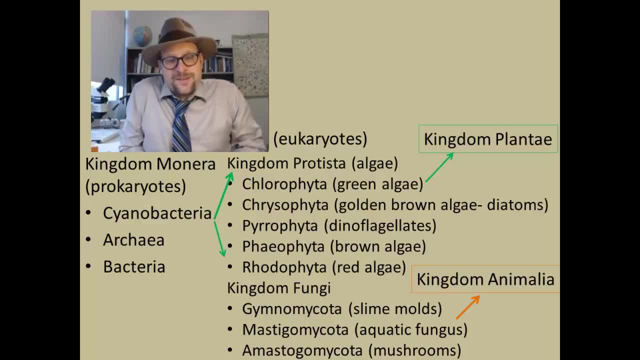 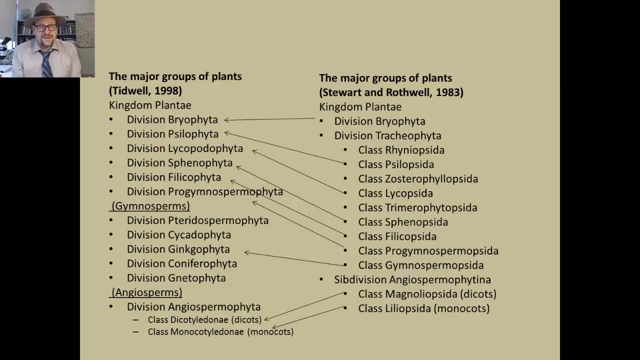 most closely related to animals, And so that is kind of where these things sit. We will talk about the algae next week, and we will also talk about the fungi and the fossil record of fungi. in a separate lecture I mentioned that plant systematics is debated. 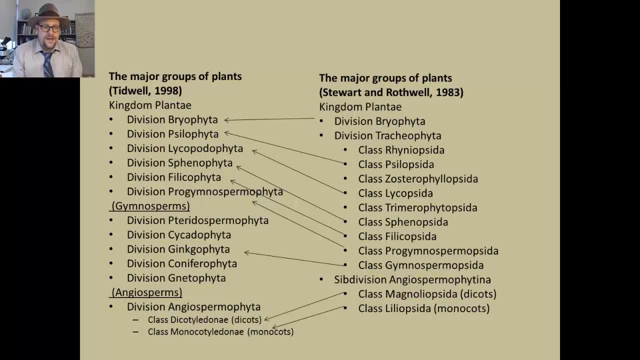 Here is a classification of plants from the Stuart and Rothwell book and what William Tidwell lists in his Paleobotany book. Many of the names and the ranks of those names are different. We will try to use the names listed in the Stuart and Rothwell book, but don't freak. 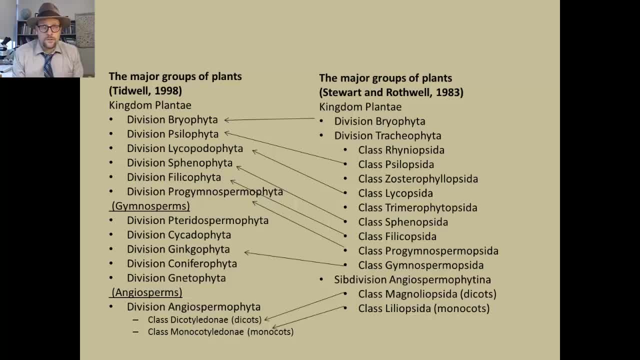 out if I slip in some different names for the various groups. Note that most of the Tidwell names are different. They end with "-phyta", while the Stuart and Rothwell classified many of these groups within the classes, and then end in "-opstia". 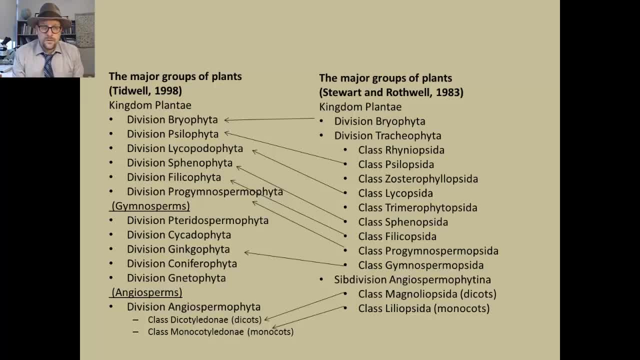 So, basically, the endings are slightly different, and so the Tidwell is a little bit more modern, and so we will be using both of these terms. but I will just kind of help clarify it. We will try to stick with what we are using in our textbook. 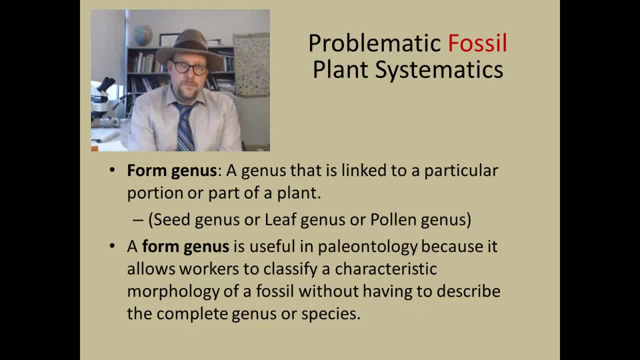 All right. Finally, we have the very practical problem, The problem of form taxa, That is, a name or a genus that is linked to a particular portion of the planet, For example, a seed genus or a leaf genus or a pollen genus. 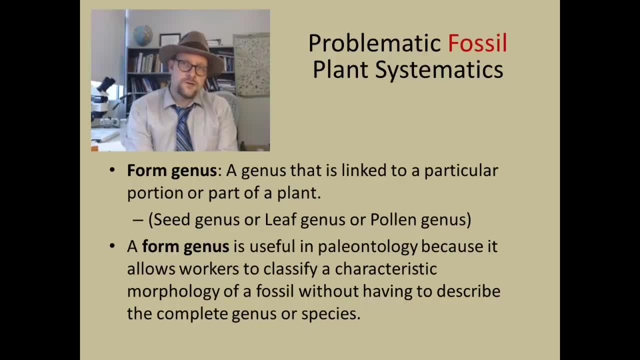 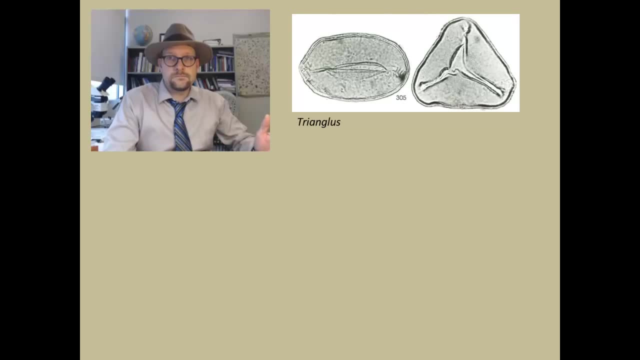 This is useful to paleontologists because it allows for classification without having to know the complete parts of a plant, but can be very confusing to students. Here is a hypothetical example. Imagine that you are studying fossil pollen and you find a form of fossil pollen and 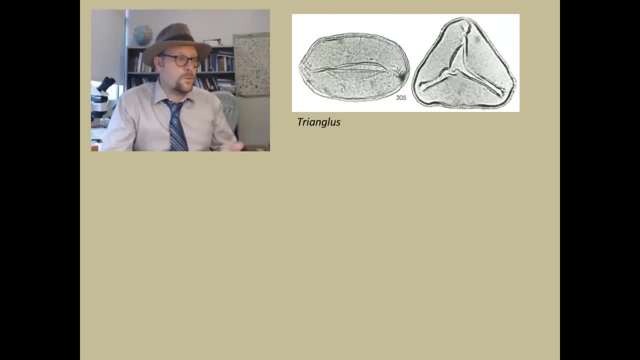 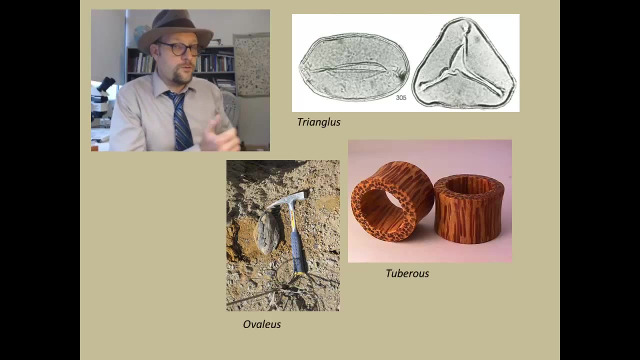 you name it Trangulus. Another worker could be working somewhere else and they could find a piece of wood, and hence they could come up with a name, and they call that Tuberous. Another researcher might find a piece of seed and they might name that Ovus. and finally, 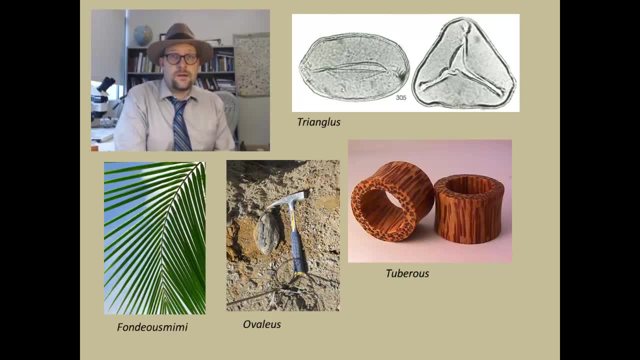 a worker might find a leaf. They could name that Tuberous, Or they could name that Ovidius decide to name that Fondiamysis mimmi. None of these workers may suspect that, in fact, all of these fossils came from the exact 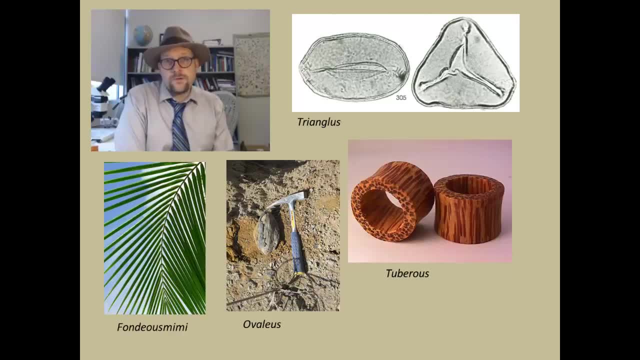 same plant, lest they found them all together and preserved, which is kind of rare, Or what they might suspect is that they came from the same plant is if they are closely related to a living form that has this type of pollen and wood and seed and leaves. 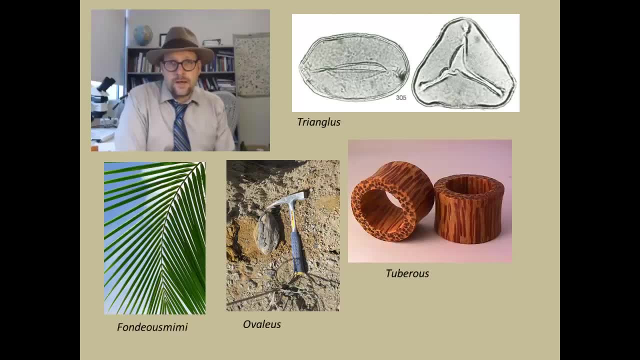 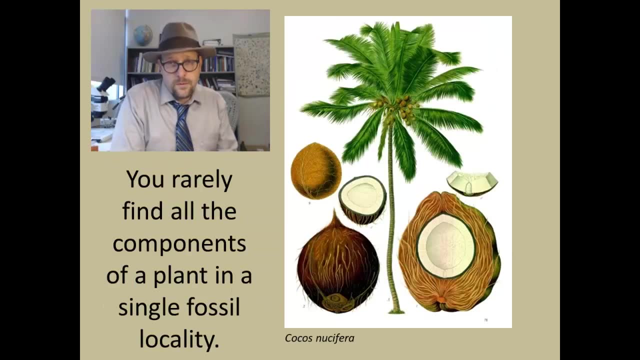 And so then we would know that they all come from that type of plant. For this particular plant, they all come from the coconut palm, Cocos nefraria, a true biological species. So you rarely find all the components of a plant at a single fossil locality, so form. 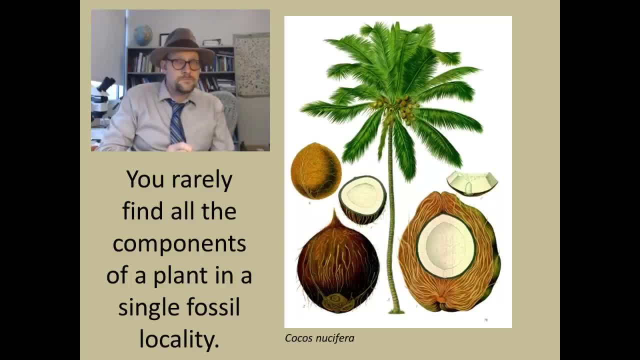 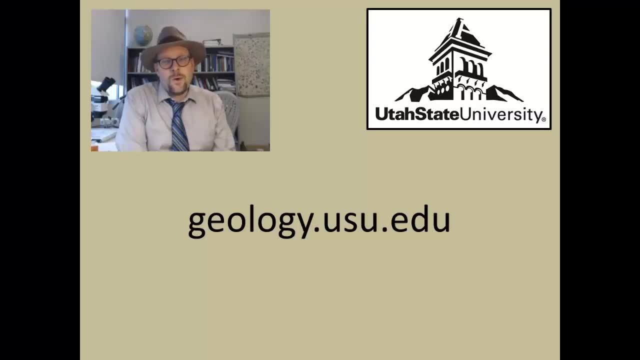 tacks are useful, but they can be problematic as well. These are some of the problems. Thanks for watching another lecture video. If you are interested in taking a course at Utah State University in geology, check out the geology website at geologyusuedu. 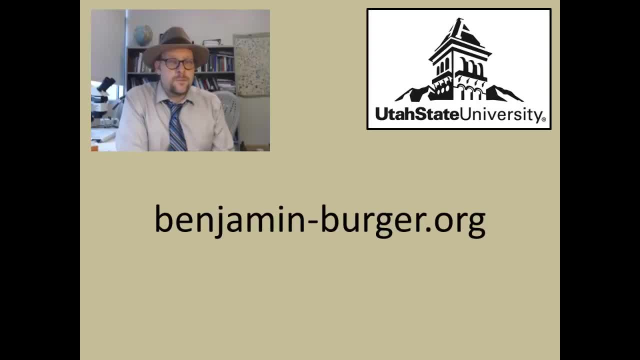 And if you are interested in who I am and the research I do, check out my website at benjaminslashbergerorg. Thanks again for watching another lecture video.